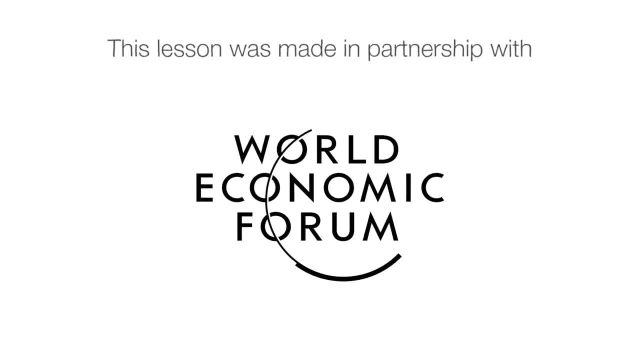 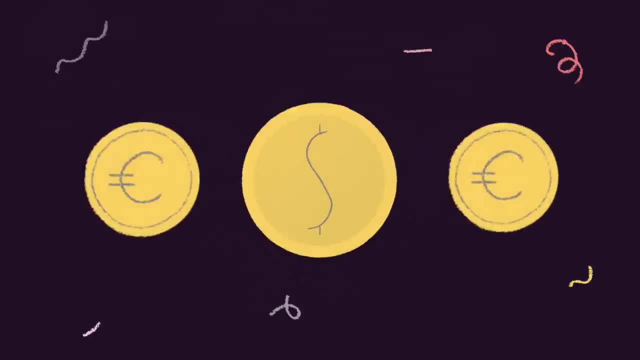 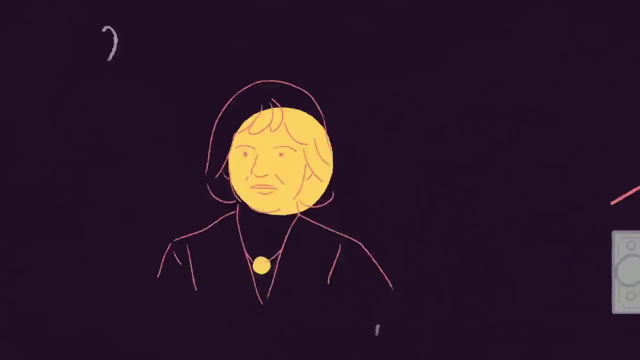 What does it mean for a country to have a healthy economy? What does a healthy economy even look like? Does it look like this? What about? like this Economist, Kate Raworth shared a pretty interesting answer to this question on the TED interview podcast and it challenges. 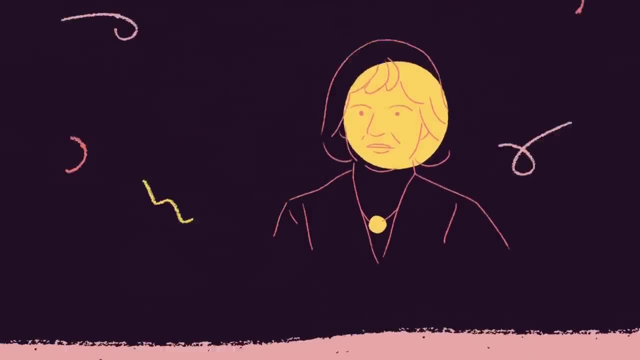 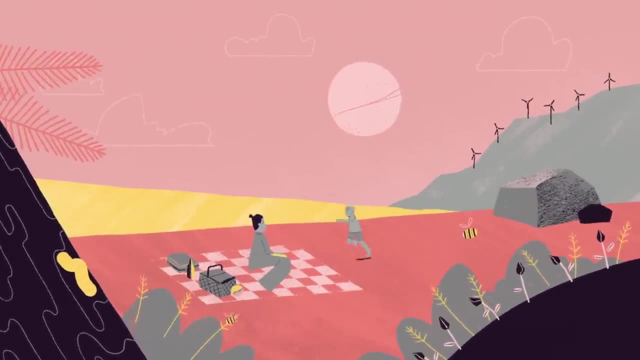 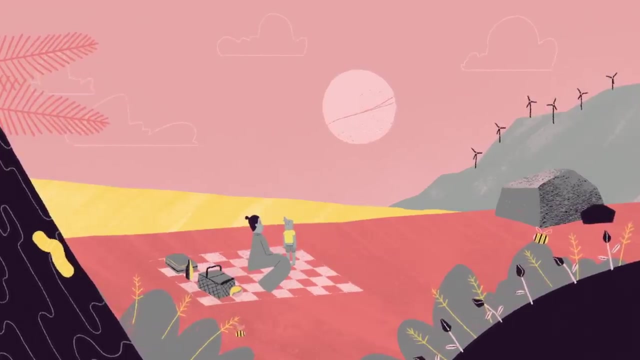 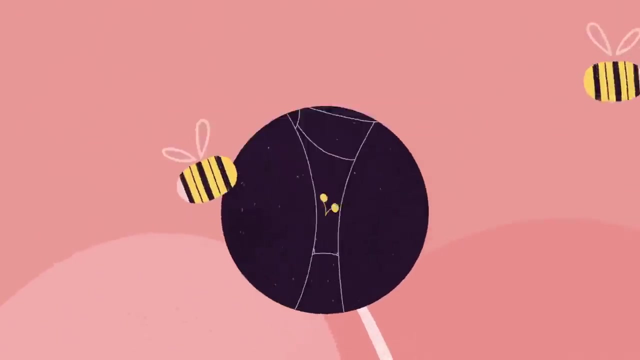 an idea that most economists take for granted. We live, particularly in the West, particularly the last 150 years, in a society that has a very strong belief that growth is the sign of progress, And to a certain extent it's true. We love to see our kids grow, We love to see nature growing in spring. Growth is 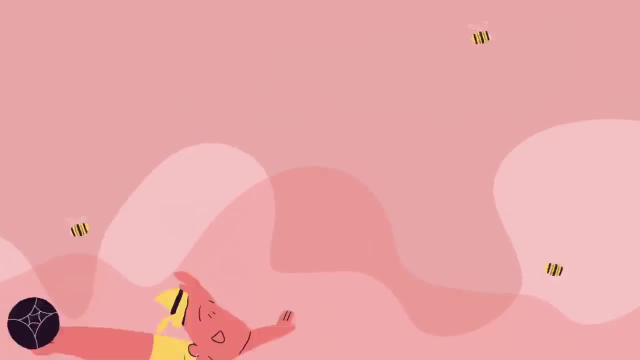 a wonderful, healthy phase of life. But in our economies it's like we've turned to Peter Pan economics, the economy that never wanted to grow up. It wanted to grow and grow and grow forever. And it becomes this permanent phase, But we 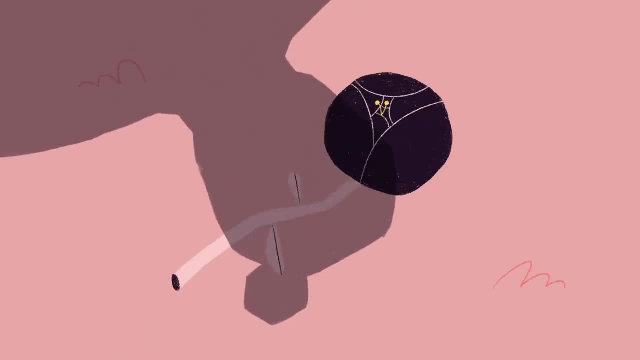 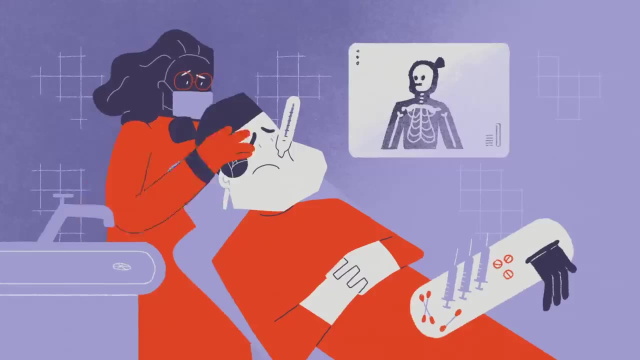 already know in our own bodies, in our own lives, that there's another side to this metaphor of growth that we love so much. If I told you my friend had gone to the doctor and the doctor told her she had a growth that already feels completely different, Because in the 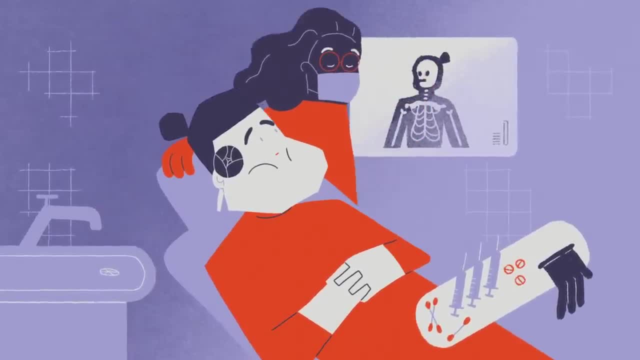 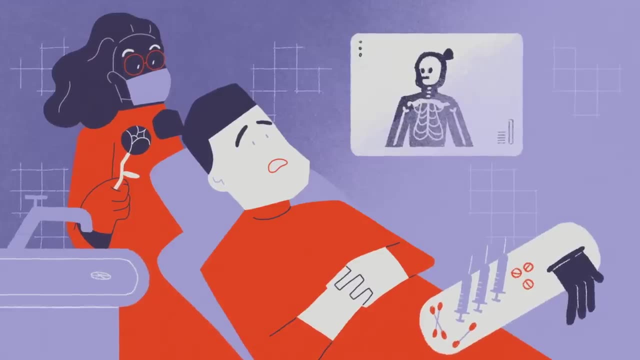 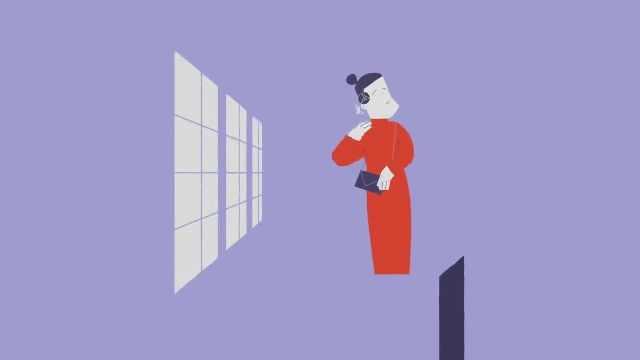 space of our own bodies. we know that when something tries to grow endlessly within this healthy, dynamic living, It is a threat to the health of the whole And we do everything we can to stop it. But when we step into our economies, for some reason we think that endless growth is progress. 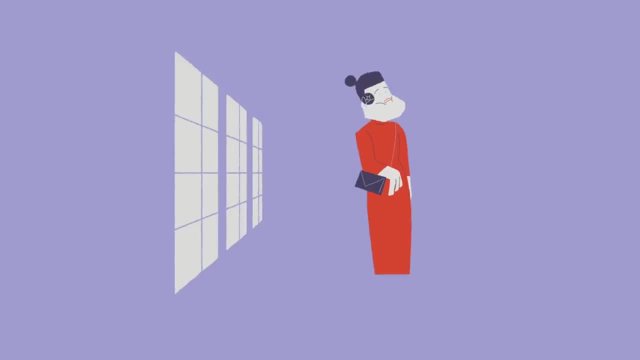 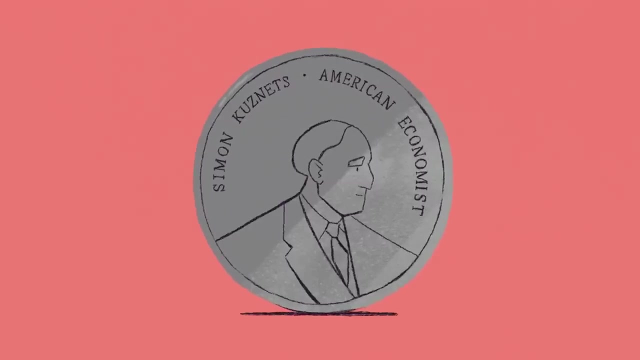 And we are now running into severe problems because we are addicted to endless growth. Simon Kuznets: he was asked in the 1930s by US Congress to come up for the first time with a single number to measure the output of the economy. America could say: well, we. 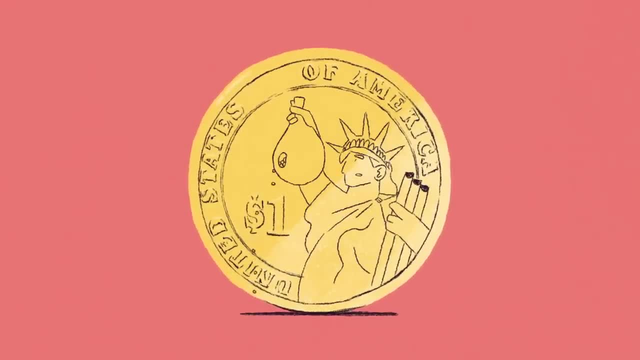 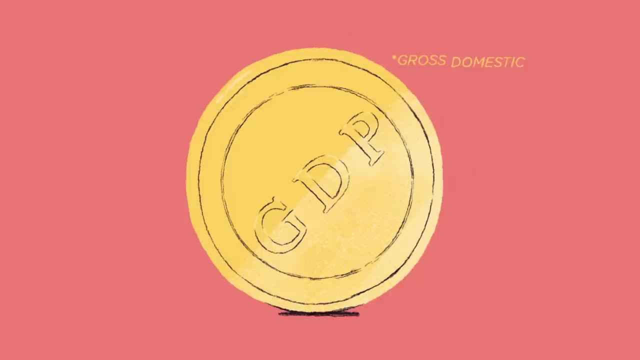 produce so many tons of steel and so many bags of grain, Can we add it all together? So they commissioned him to do this And he said: yes, I can. I can add it all together in one number: National income, what we now know as GDP. But he gave. 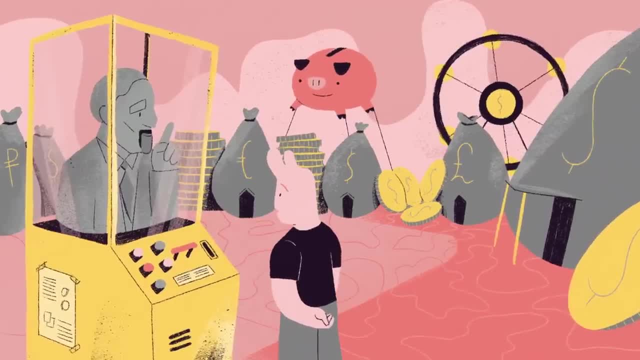 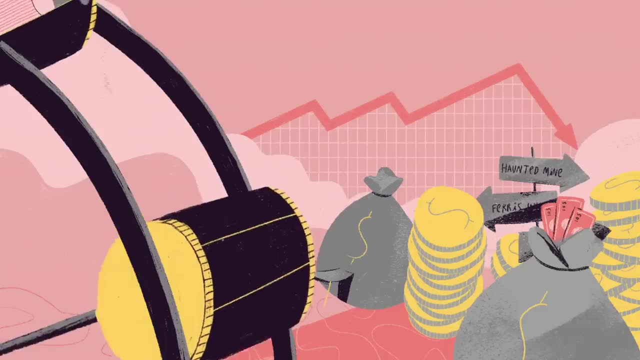 it with a caveat. He said the welfare of a nation can scarcely be known from this number. Don't mix it up with welfare, right, Because it tells us nothing about the unpaid caring work of parents. It tells us nothing about the value that's created in communities, because 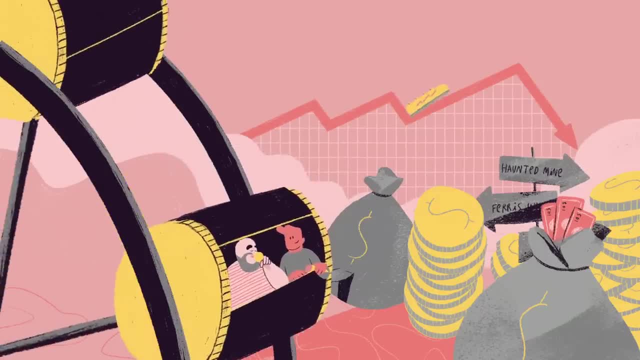 that's not price And it's a measure of the flow of economic value. It tells us nothing about the living world, the forests, the mines that get run down. It tells us nothing about the value that's created in communities, because it tells us nothing about the living. 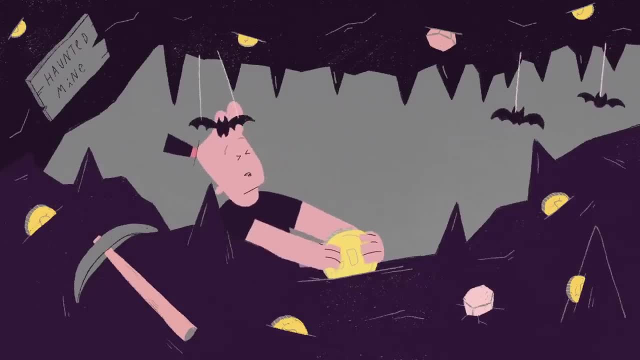 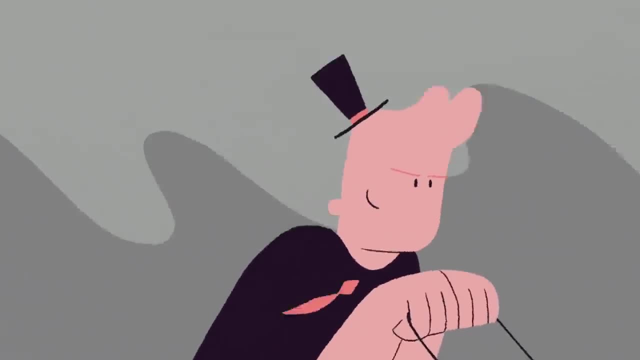 world, the forests, the mines that get run down in order to create this value. But the convenience, the temptation of this single number was so great that politicians sort of tucked it in their armpit and carried right on And we ended up in a horse race. 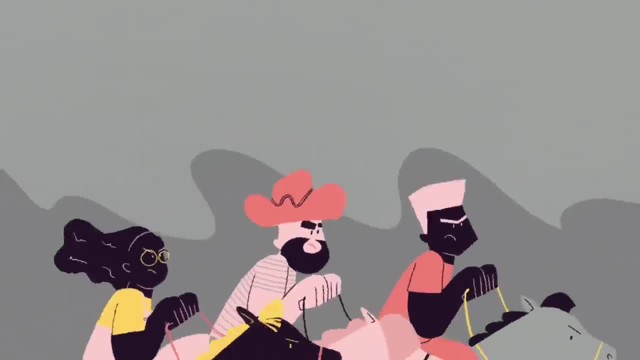 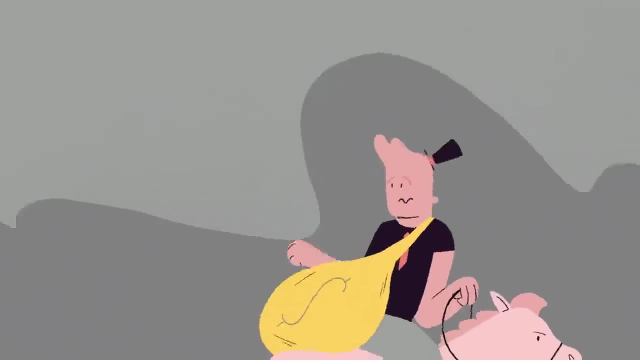 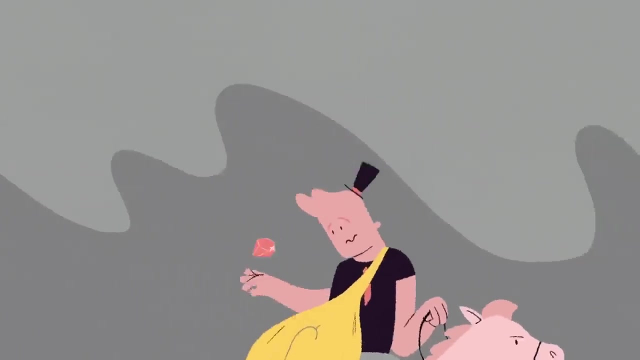 of pursuing GDP growth. The dream is that GDP can keep on increasing, We can have increasing financial returns, but that we can decouple from using Earth's resources. We can use less carbon and less metals and minerals and plastics, And we can use less of the Earth's land surface and separate these two ever rising GDP and 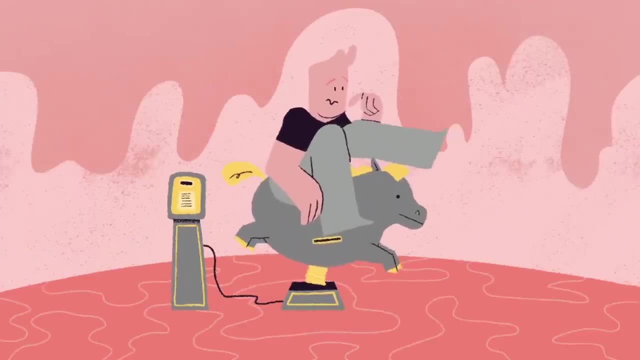 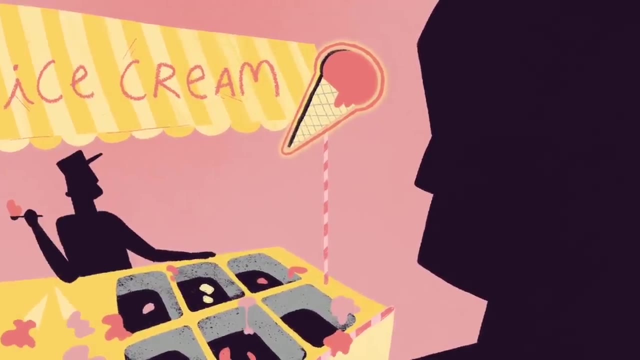 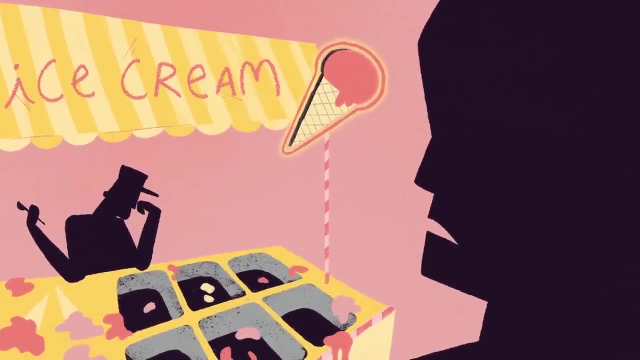 falling resource use. It's a fabulous dream, Would that it would be true. We are at a time of climate emergency, of ecosystem collapse. We need to radically reduce our use of Earth's resources, And we're nowhere close to that. So I offer it as a compass for 21st century. 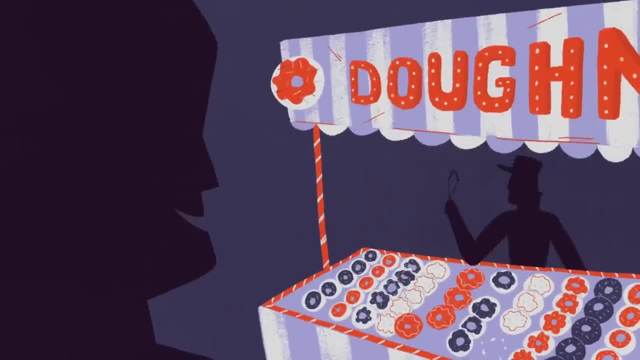 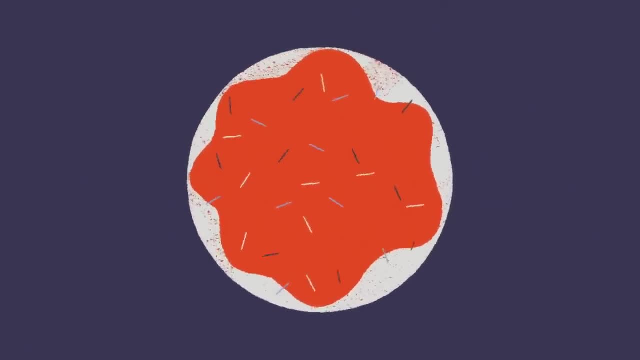 prosperity And this compass, silly though it sounds, it looks like a donut with the hole in the middle. So imagine, from the center of it, humanity's use of Earth's resources radiating out from the middle of that picture, So in the hole in the middle. 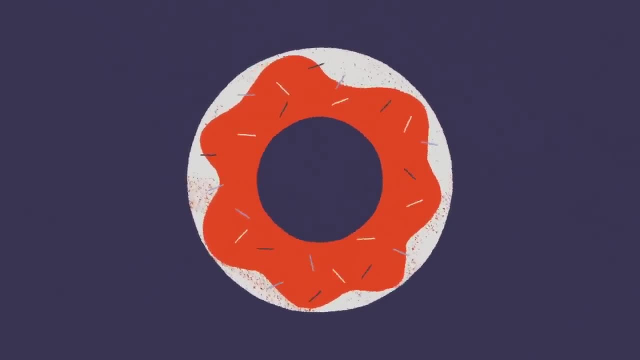 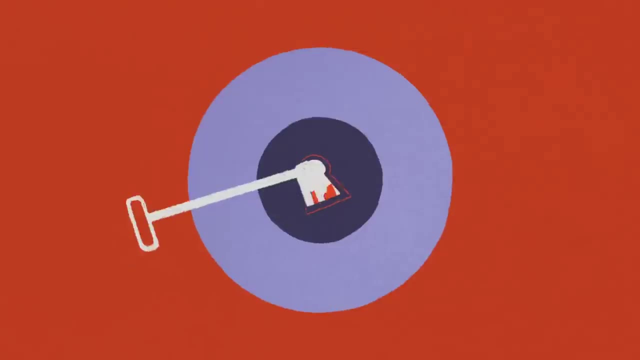 of the donut. that is the place where people don't have enough resources to meet the essentials of life. It's where people don't have enough food or healthcare, or education or housing or gender equality or political voice or access to energy, And we want to leave nobody in. 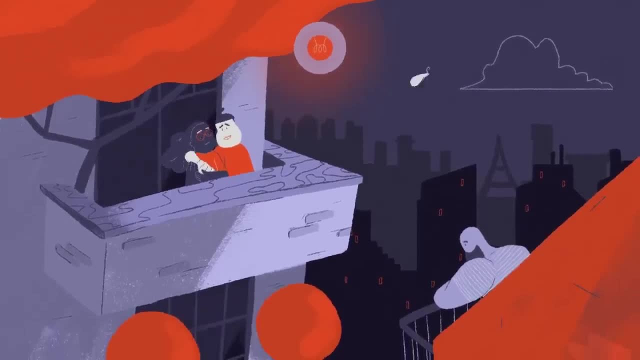 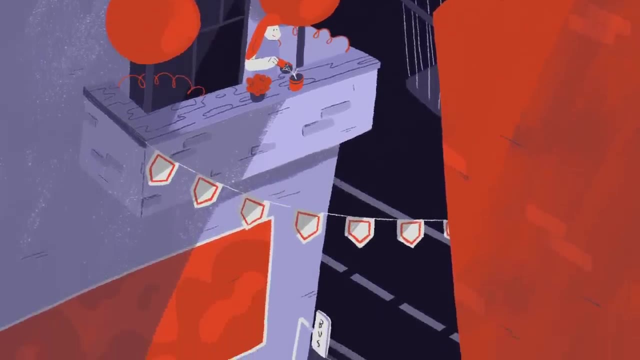 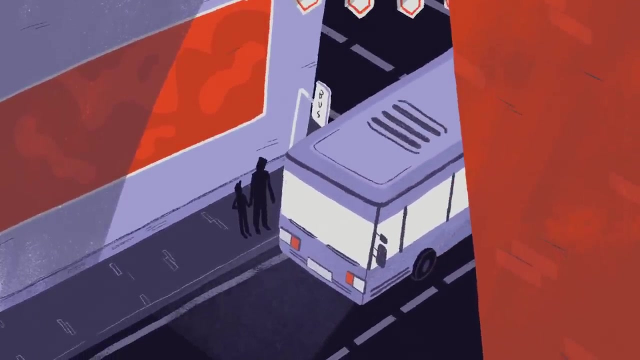 that hole. We want to get everybody over a social foundation So all people on this planet can lead lives of dignity and opportunity and community, And in low income countries it absolutely makes sense. Yes, let's see the economy grow in ways that invest in health and education and transport. for all, That was a very 20th. 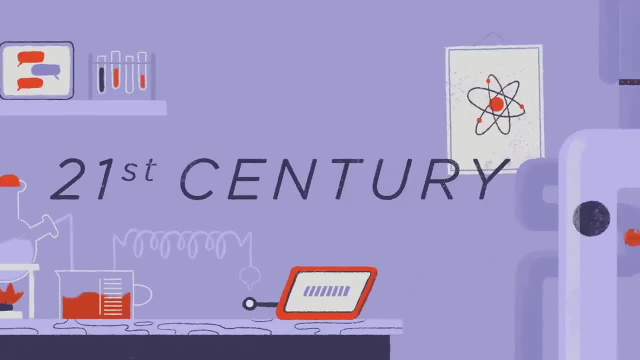 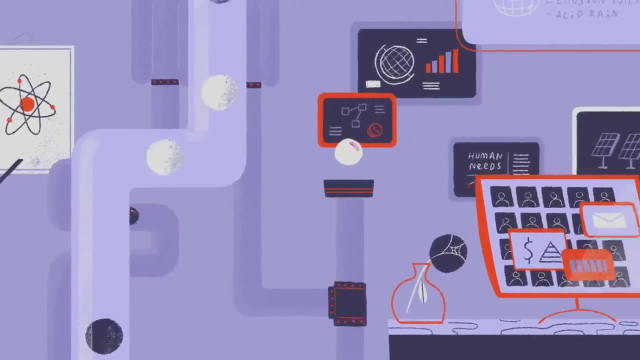 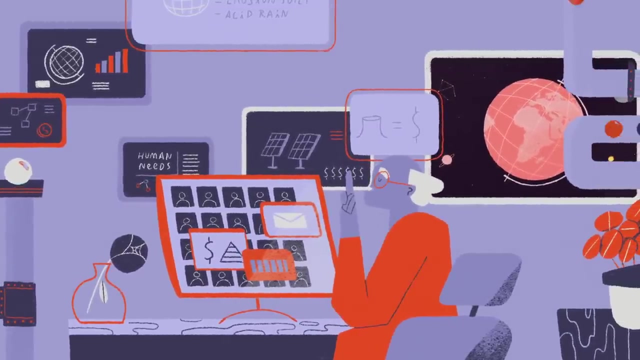 century project. We're in the 21st century. We have Earth system scientists who started looking at the impact we were having on the climate and the loss of soils and acid rain and the hole in the ozone layer and the collapse of species And they said: hang on, we've been ignoring our planet in the growing to meet human needs.